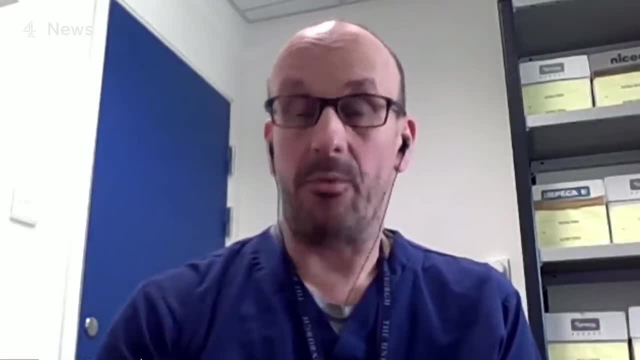 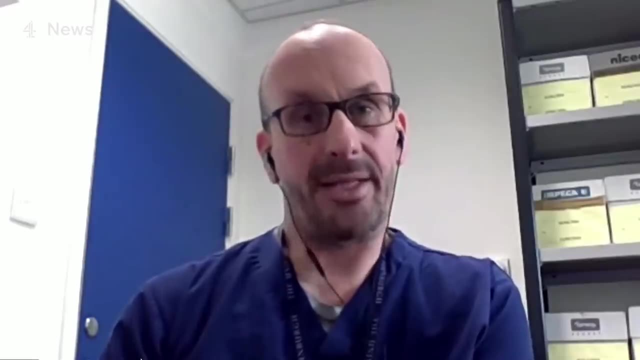 to every household and said: look after it, be safe with it, don't let anyone get close to it. And imagine having 40 years that bottle of sarin sitting in all those cupboards. and that's the equivalent of what happened by handing out these pesticides. It's really that dangerous. that is a valid equivalent: sarin. You know we have pesticides which are a thousand times safer, 10,000 times safer than those compounds. Accidental ingestion, suicide, tens of thousands of Gramoxone deaths. 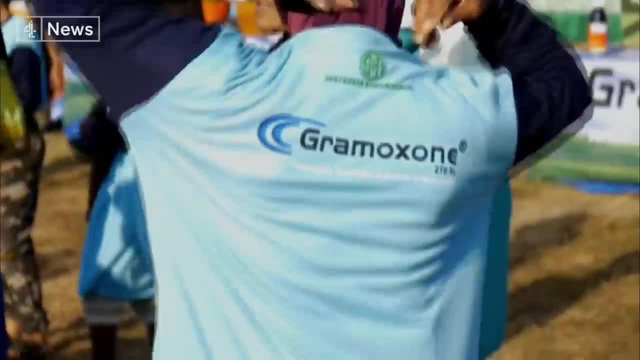 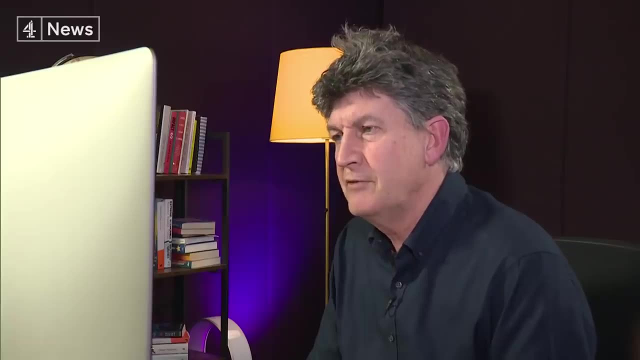 Some UN experts say it is hundreds of thousands. It's been on the market for decades, despite countless thousands, hundreds of thousands of deaths around the world. You've called it the worst of the worst. Indeed, It is one of the most acutely toxic pesticides that's on the market. 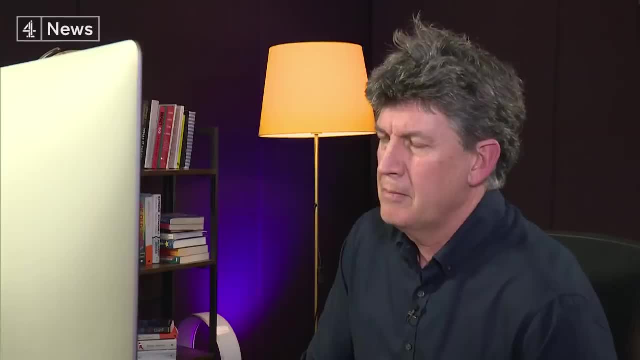 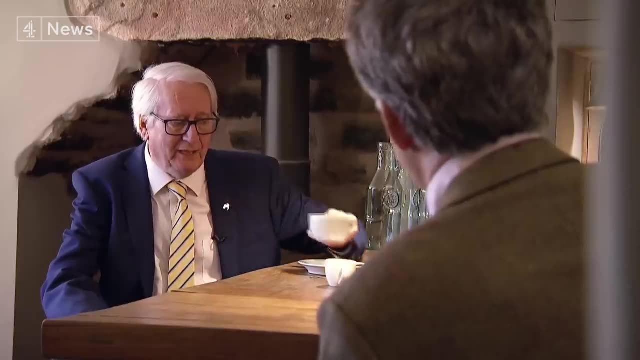 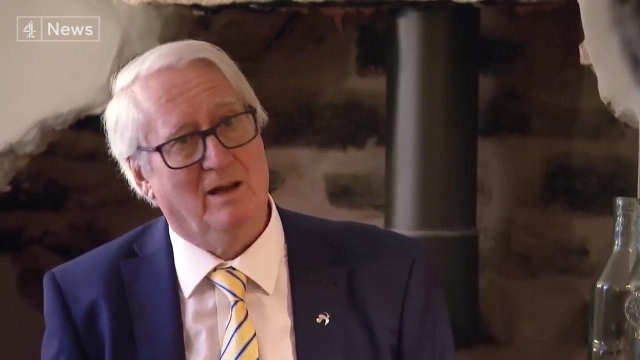 market just a few tablespoons is deadly, and equally concerning is the vast volume of exports that are coming out of the UK. we've come to Derbyshire to meet Professor John Haylings. well, tell you what, Alex, I can't sleep at night at the moment because this has reached. he's finally going public about Gramoxone. 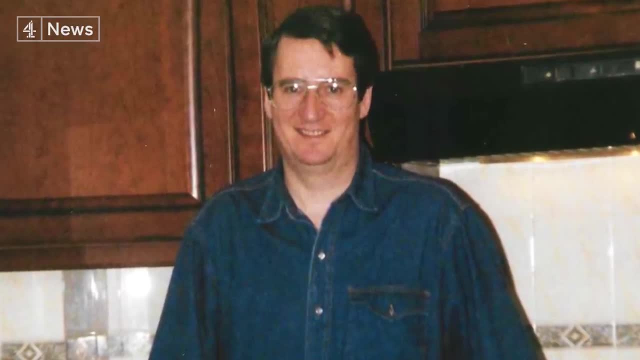 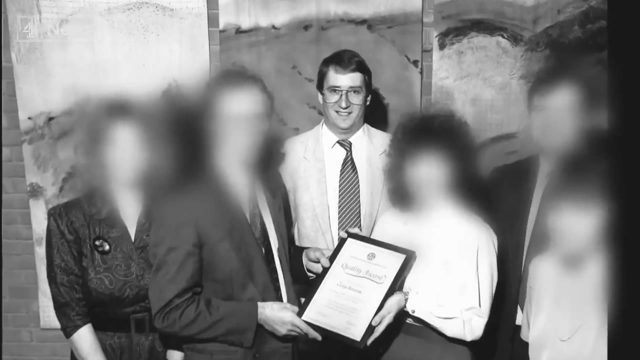 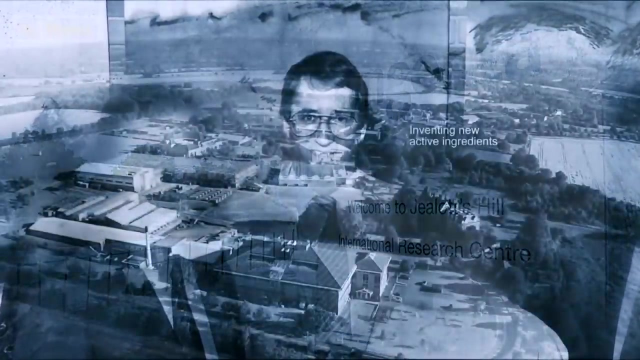 after almost half a century of trying to force the industry to make it safer. it's the same what has happened over the last 40 years, and they're still dying. the story begins decades ago at Jellett's Hill, Syngenta's Berkshire research base. 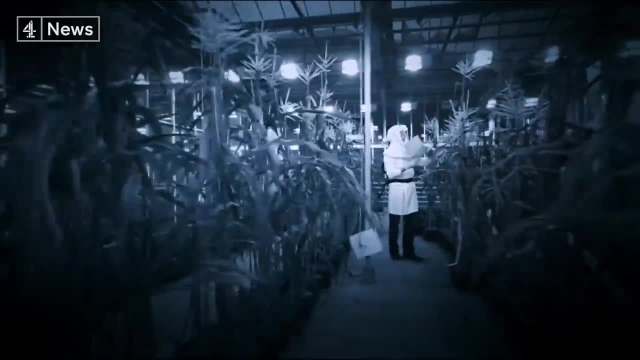 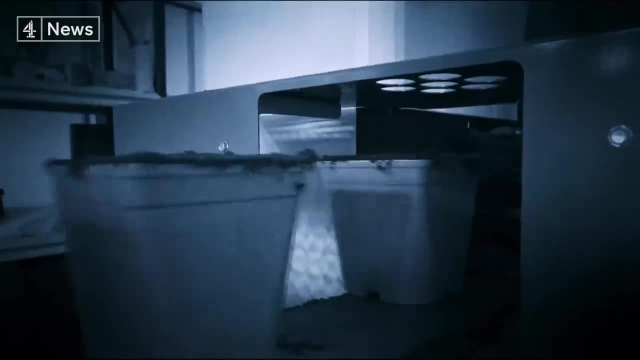 as far back as the 1970s. its predecessor company, ICI, wanted to put an emetic, a vomiting agent, into Gramoxone to try and make it safer. secret company documents never made public till now, show that by the late 1980s the company was still in the process of making it safer and the 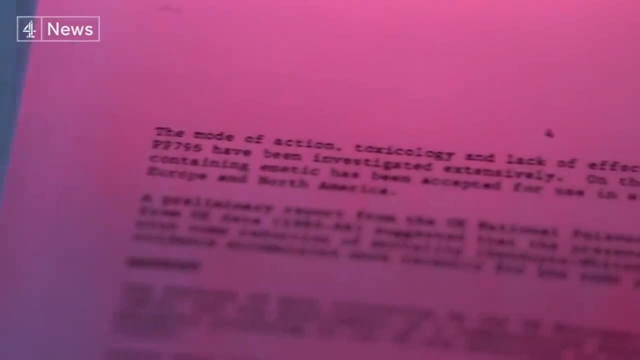 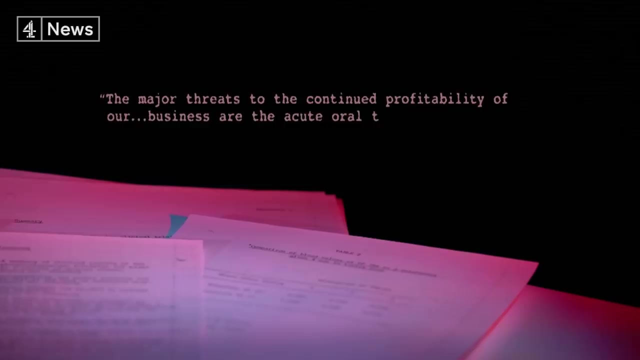 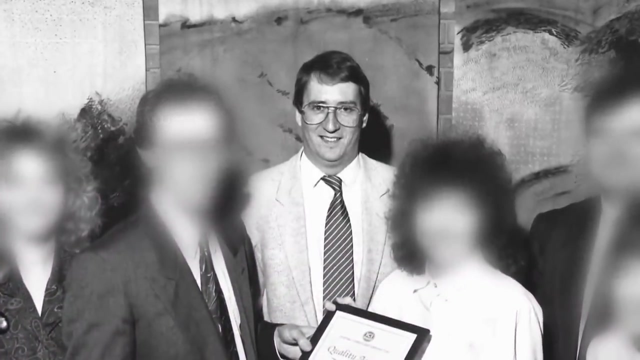 80s they feared it was so lethal, everyone would just ban it. the major threats to the continued profitability of our business are the acute oral toxicity and the external perception that this gives the product. long before that, John Haylings had been called in to try to make Gramoxone safer there'd. 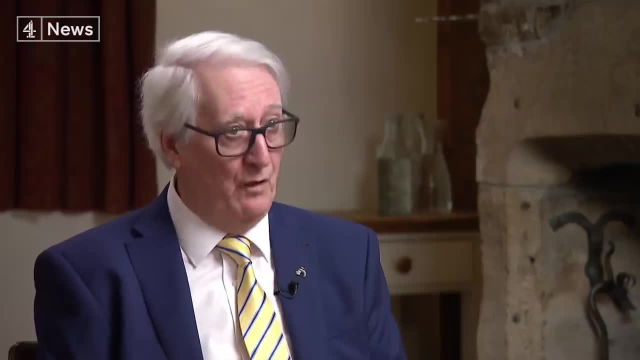 already been a recommendation of increasing the emetic by five-fold, even before I had even started. more than 40 years ago, the company had been called in to try to make Gramoxone safer. there'd already been a recommendation of increasing the emetic by five-fold even before I had even started- more than 40. 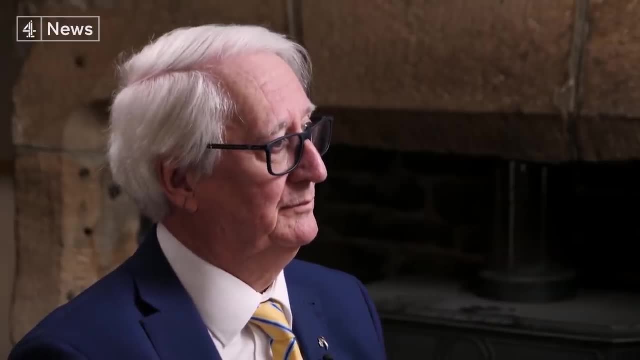 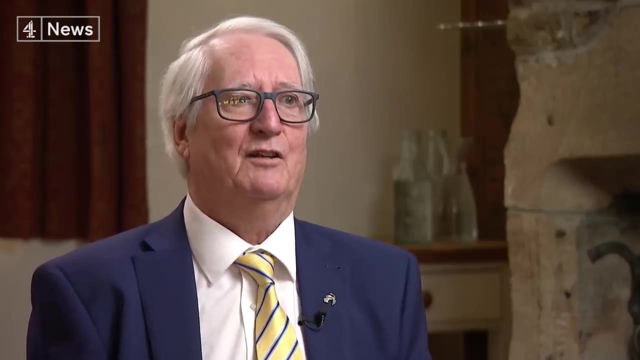 years on, after tens of thousands more deaths, John Haylings had another meeting with Syngenta, the company he used to work for, and left on good terms. I think there was a lot of them jaw-dropping in that meeting, a lot of the new people on. 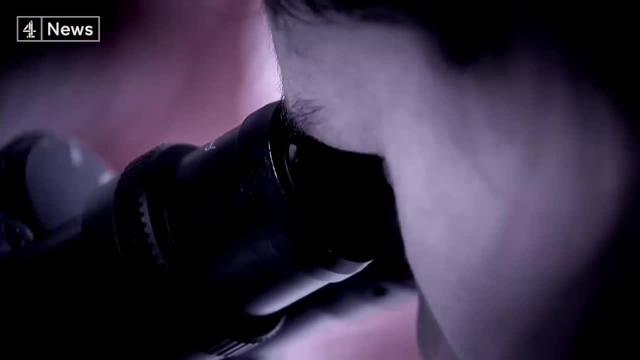 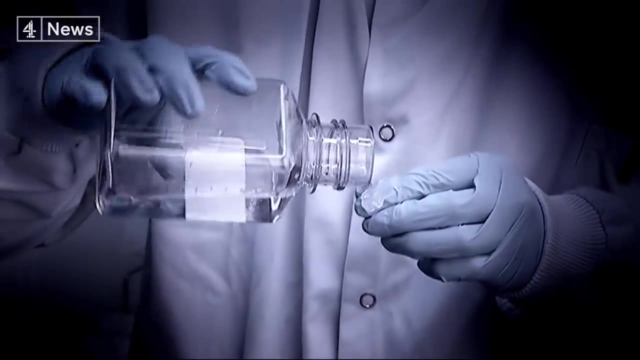 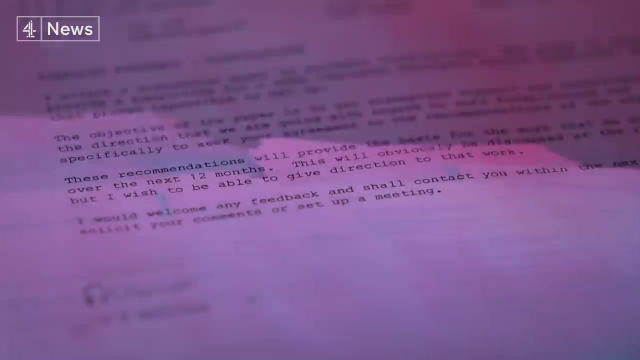 the block did not know that there'd been a big problem. but tonight we can reveal that for all those decades Syngenta and its predecessor companies had safer versions on the shelf ready to go, but only if Gramoxone got banned. a memo from way back in 1990 reads: much work on safer formulations has already. 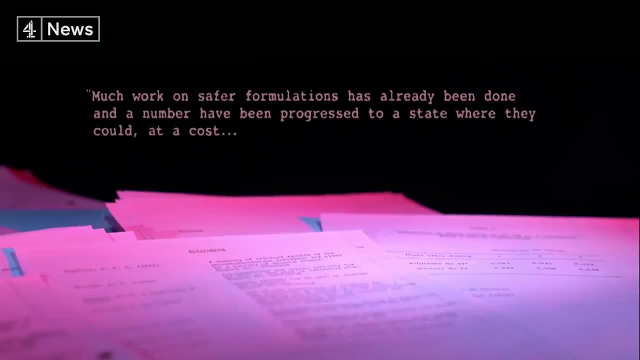 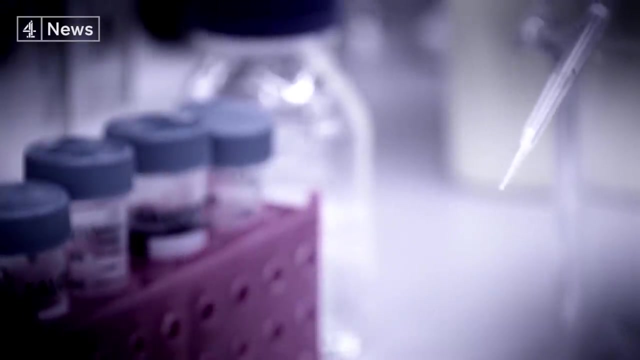 been done, and a number have been progressed to a state where they could, at a cost, be introduced to markets, and this would provide a basket of options to offer when faced with a regulatory crisis. in plain English, we can stop the mass death, but only if we face a ban. Syngenta inherited this policy when it took over production in 2000 and it was the first time that Gramoxone had ever been banned in the United States in 2000, and it was the first time that Gramoxone had ever been banned in the United States in 2000, and it appears that it has followed it for 21 years. John Hayling says it all comes down to money. 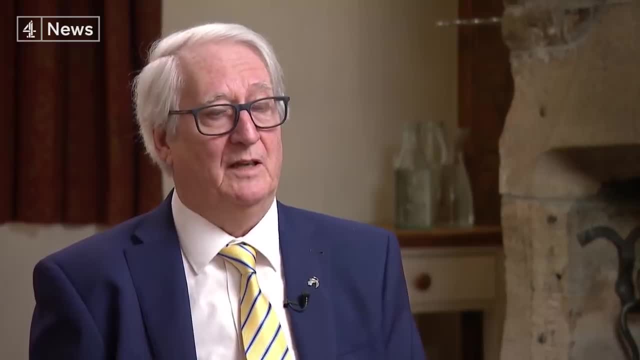 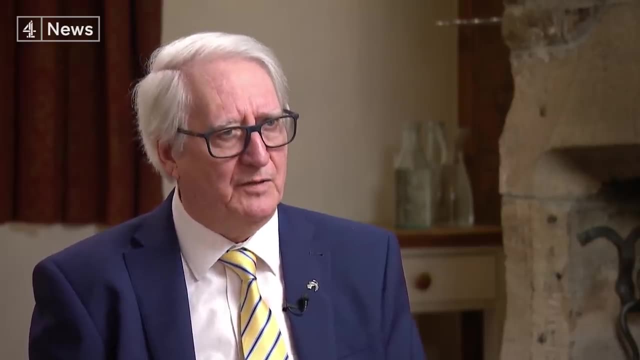 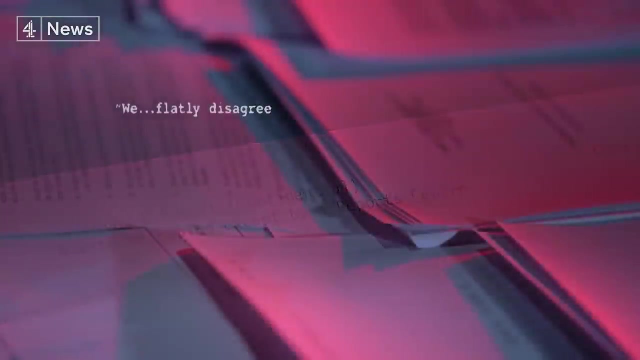 undoubtedly the the profit before safety. I think is a trend that has gone on in a lot of industries, but here you're talking about people's lives. just two years ago, a senior Syngenta executive wrote: we flatly disagree with any suggestion that in developing this product, we should be able to provide a 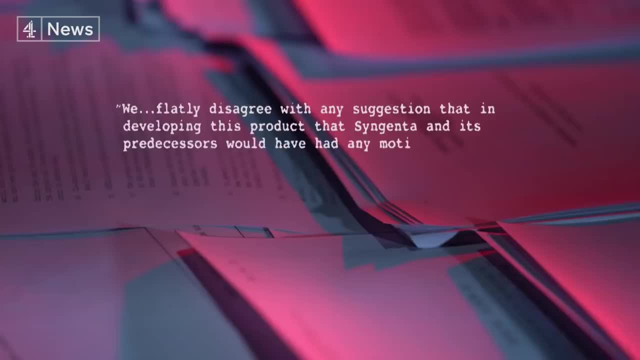 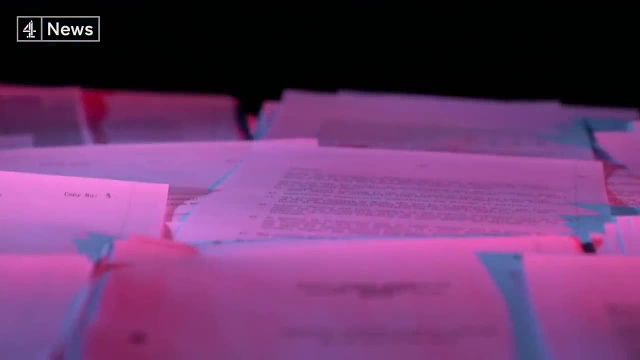 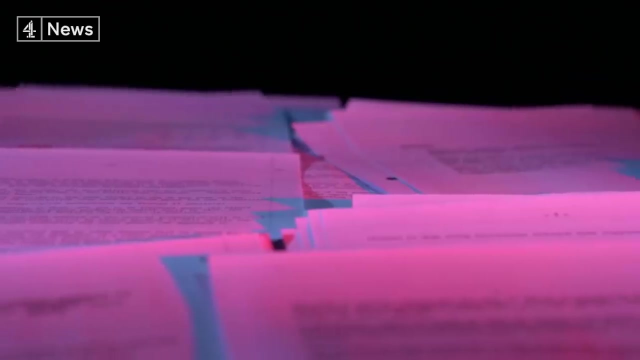 product that Syngenta and its predecessors would have had any motive other than to best address the ingestion risk. but Greenpeace unearthed public eye and this program now have a slew of secret company documents never made public until tonight. they prove Syngenta's predecessor companies refused 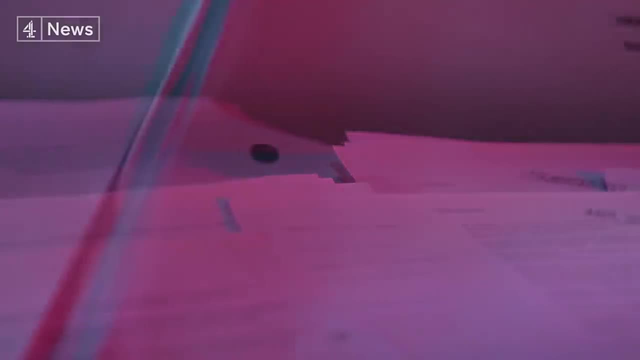 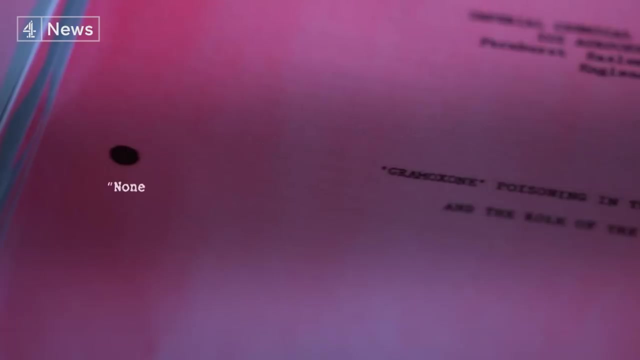 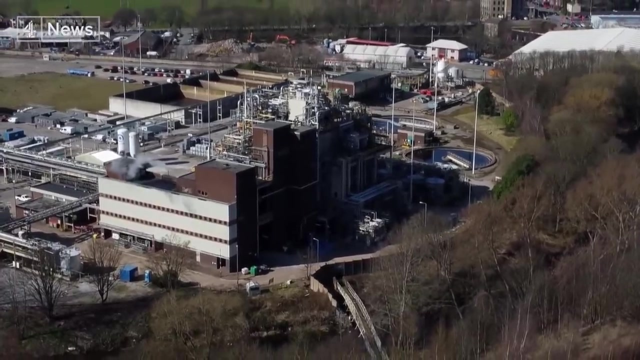 to make Gramoxone safer because it would be too expensive. the introduction on a global basis would destroy group profit and none of the alternative formulations currently available offer an economically acceptable solution to the suicide problem. so Syngenta's claim two years ago that money has nothing to do with the failure to make Gramoxone? 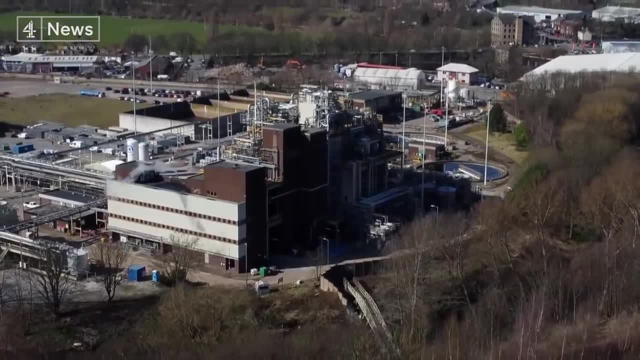 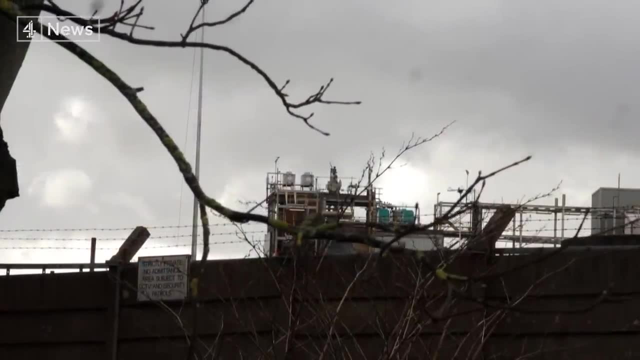 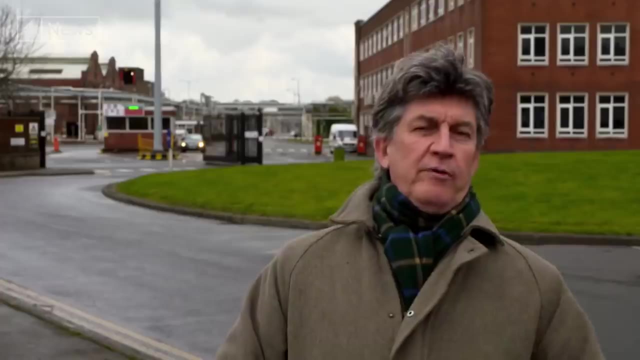 safer is false. they say they've spent hundreds of millions of dollars trying to make the product safer- definitively not. the behavior of a company driven by cost- and they stress it- brings farmers enormous financial and environmental benefits worldwide. for almost 50 years, Syngenta and its predecessor companies 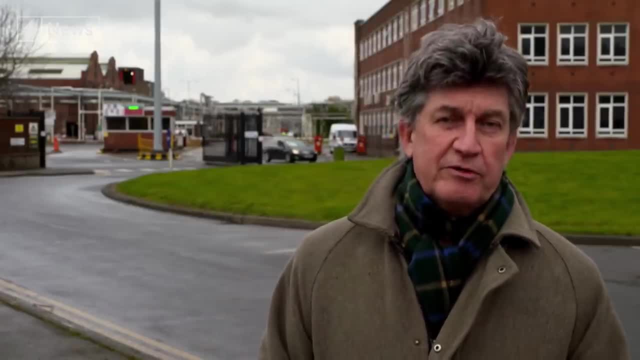 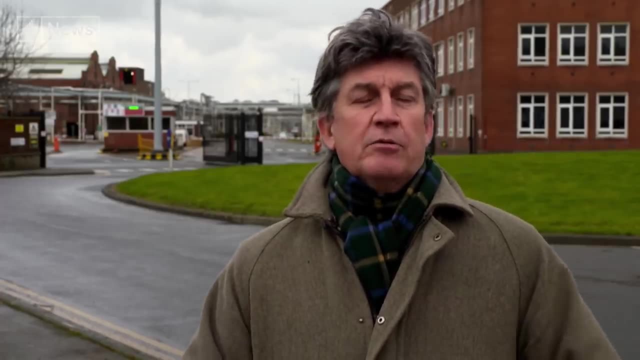 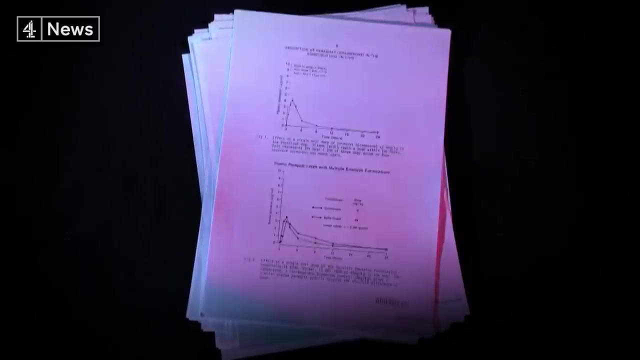 have relied on data to persuade the global safety watchdog that Gramoxone was safe, even though thousands of people continue to die. tonight we can reveal that that data was flawed and they knew it was flawed. the secret company documents spanning decades prove even the scientists producing that data used 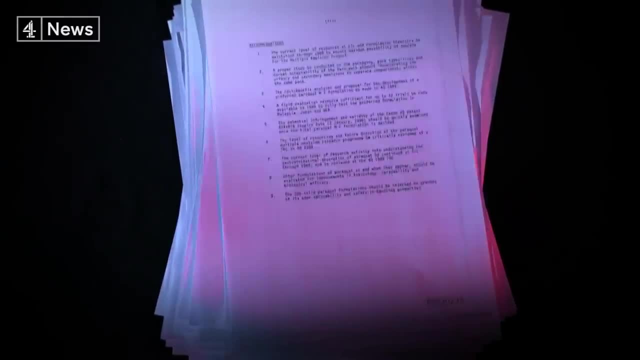 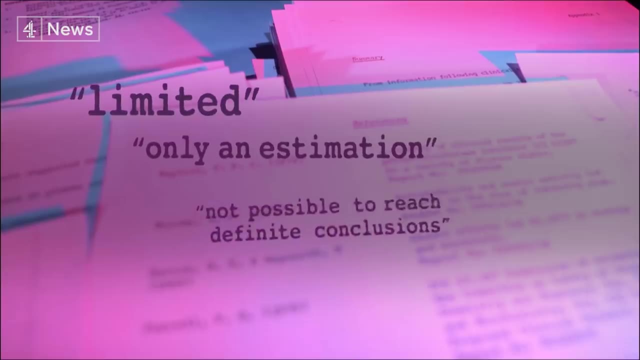 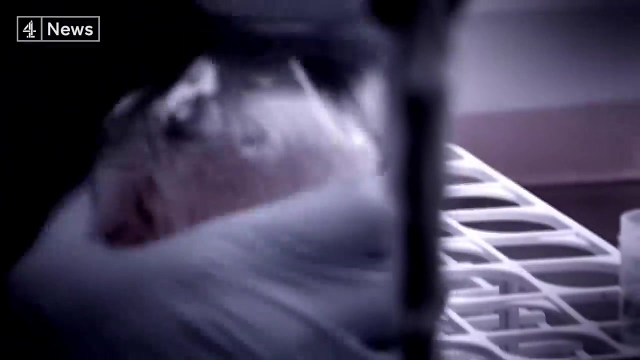 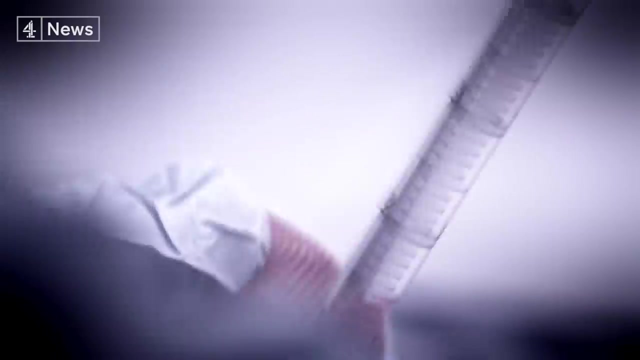 to convince the global safety regulators that gramoxone was safe were concerned. they called it limited: only an estimation, not possible to reach definite conclusions, limited clinical data, and on it goes. yet singenta's case for getting lethal gramoxone past the watchdog in 2003 was largely based on 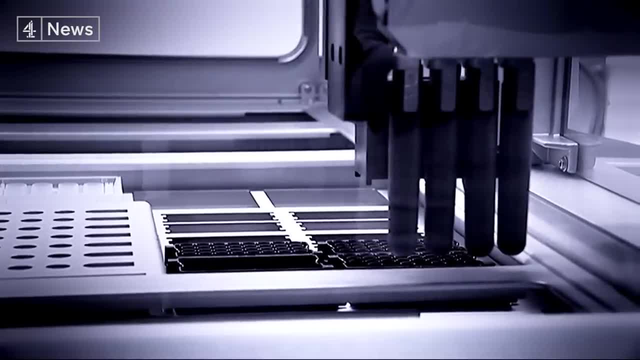 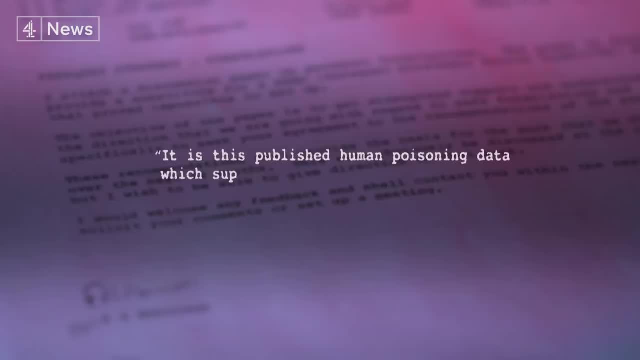 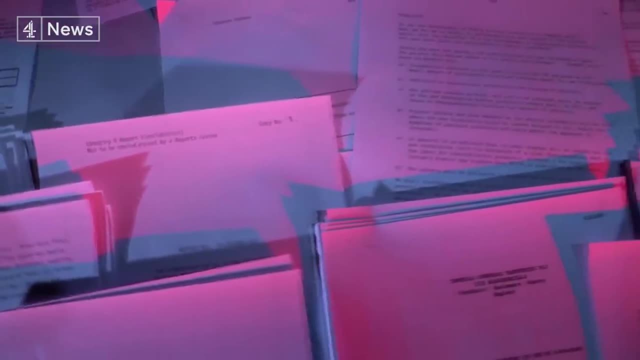 this data? how do we know? because a senior executive admitted it in 2019. it is this published human poisoning data which supports the current fao, the fao being the united nations global safety watchdog which governs herbicides. well, it seems, john haylings may finally be being. 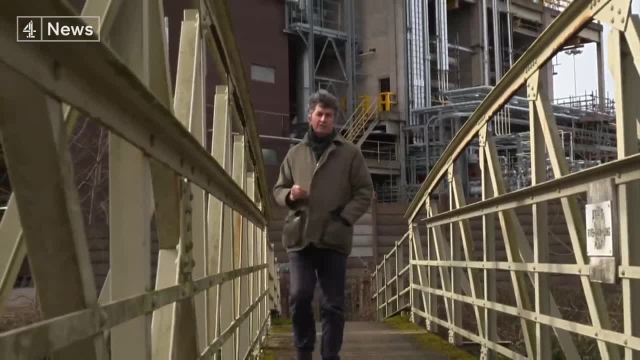 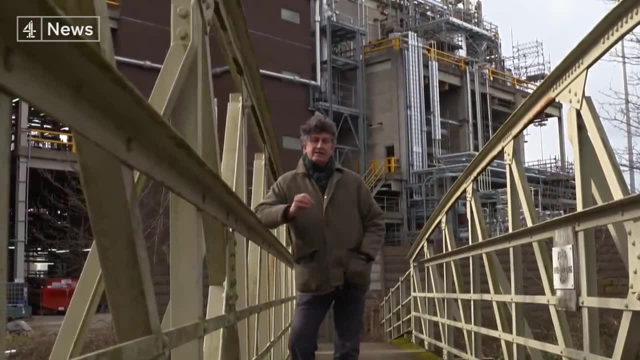 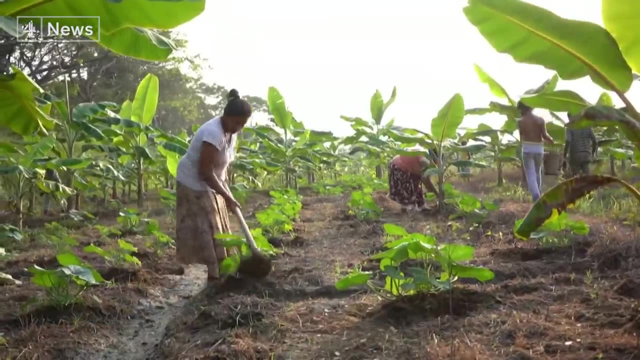 listened to at the highest level. channel 4 news has obtained a document written last year by the global safety watchdog, the fao, and in it the fao says it is now requiring singenta to make modifications to its product. all of this, of course, far too late for families in sri lanka and so many other. 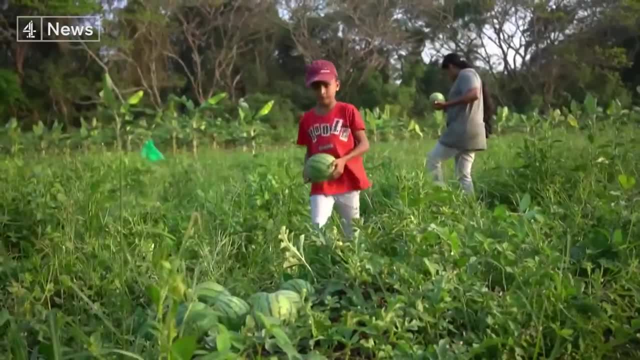 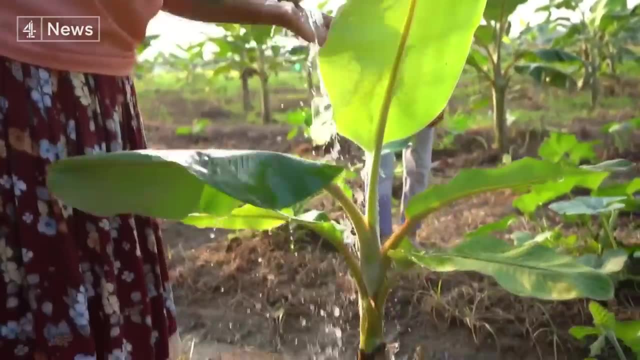 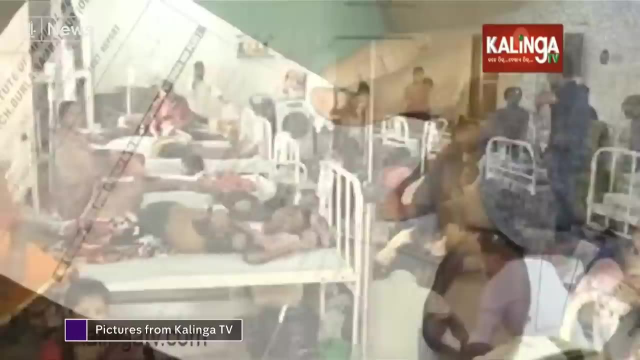 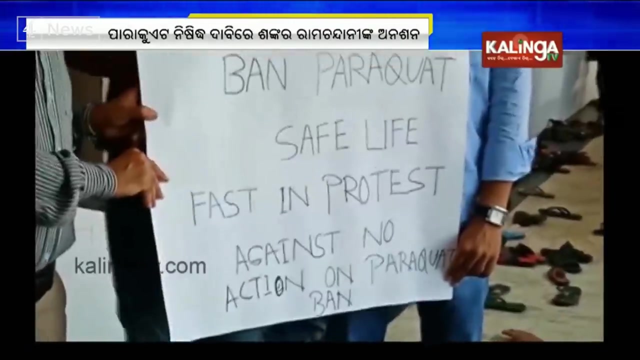 countries government finally banned gramoxone from 2008, as more than 50 countries have now done. the death rate there has dropped significantly, but many other markets remain, like india, where the death rate means gramoxone is nightly news. doctors are going on hunger strike demanding that gramoxone is banned.